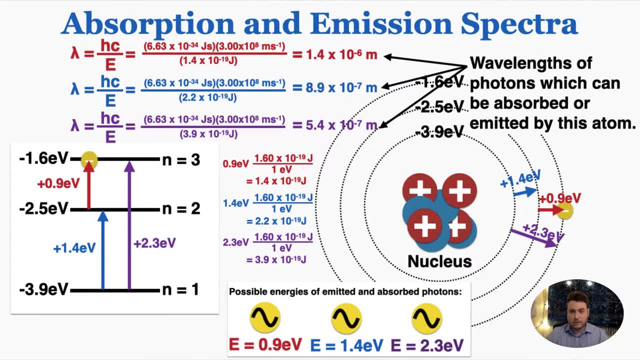 and these are what I find them to be. So these are the wavelengths of photons which can be absorbed or emitted by this atom, and if a photon that doesn't have one of those exact wavelengths interacts with this atom, what's going to happen is the photon is just going to move straight. 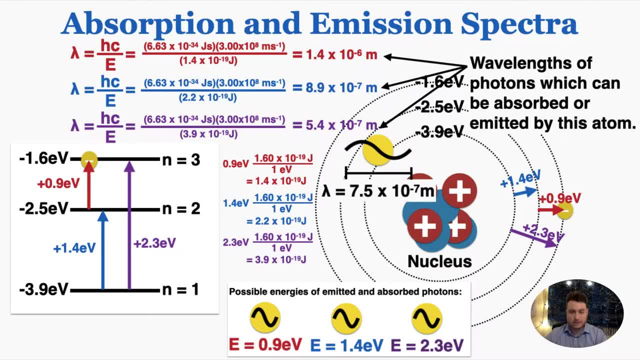 through the atom without affecting it and without being absorbed by it. That's going to be a really important concept here. This is all review. we covered this in the previous lecture, but this is going to be really central to this lecture about spectra. 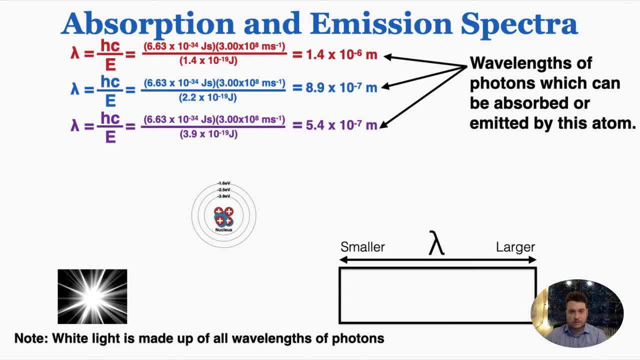 I'm going to say that we have a source of white light and some kind of detector that can detect all the different wavelengths of light that are impacting it, and white light actually contains all possible wavelengths of photons. So if we shine this white light on this detector that can 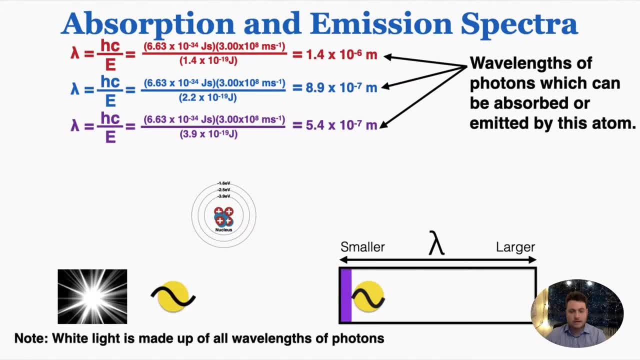 detect which wavelengths are present. this is what it would look like. The detector would record every possible wavelength of light as being present, because white light contains all possible wavelengths And in this detector we can imagine we order the wavelengths from smallest to largest, going from left to right. I'm going to shine that light on this detector again. 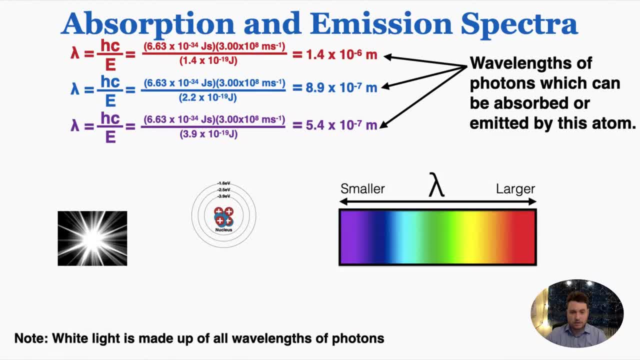 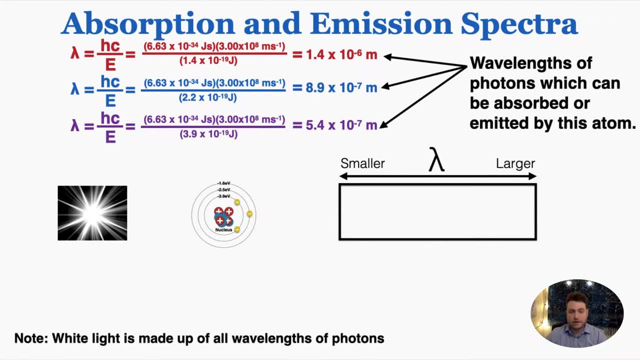 but this time I'm going to pass it through the element that we were looking at in the opening of this video. So that element is now between the white light and the detector. So what would the detector detect now? Well, every possible wavelength of light would come out of. 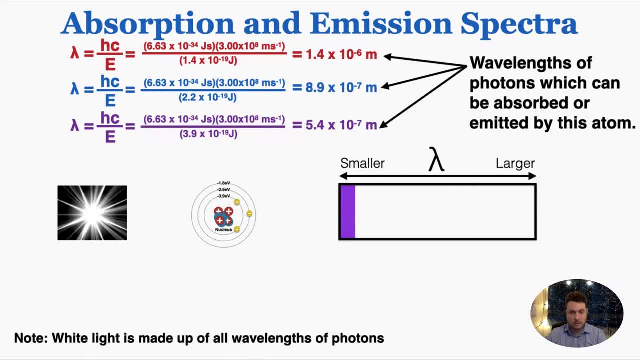 the white light source and begin to fill up our detector with all the possible wavelengths of light. But I know there are a few wavelengths that this atom can absorb, so we're going to see what happens when one of those wavelengths interacts with the atom. because, again, white light. 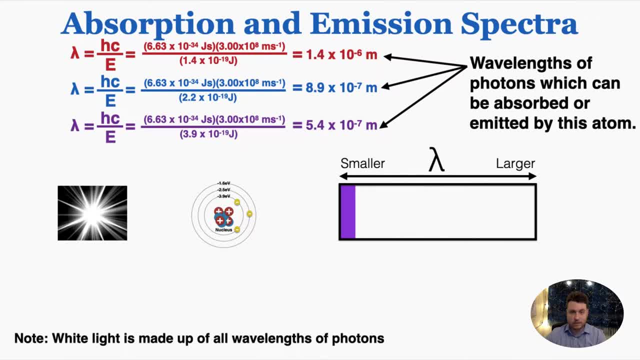 contains every possible wavelength, so it also contains those three wavelengths. If that wavelength of 5.4 times 10 to the negative seventh meters appeared, the atom could absorb this photon and it would become electron energy. So when that happens, the photon does not reach the detector. 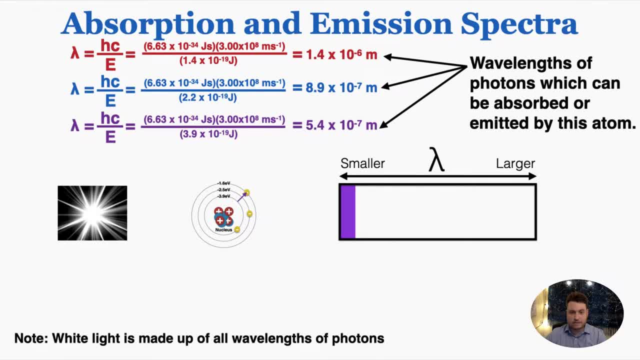 so there's going to be one very small part of our chart of wavelengths that's going to be just a black line, because no light was detected at that wavelength, because the light was kind of eaten up by the atom before it got to the detector. And if we're going to see that again, 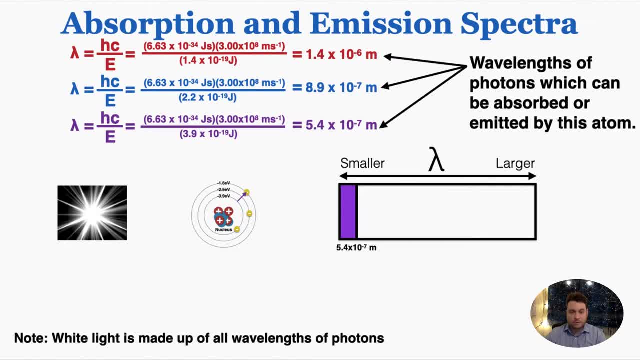 we're ordering this like by the wavelength. that black line would appear right at 5.4 times 10 to the negative seventh meters, because that was the wavelength absorbed by the atom. We can now observe the other wavelengths. Other wavelengths would continue to pass through the atom, but when we 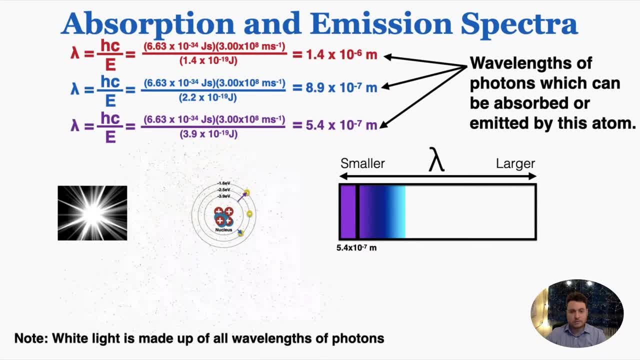 hit the next wavelength that the atom could absorb. that wavelength would also be absorbed into the energy of one of the electrons, And so again, a black vertical line would appear at that exact wavelength of 8.9 times 10, to the negative seventh meters. More light would pass through and finally, 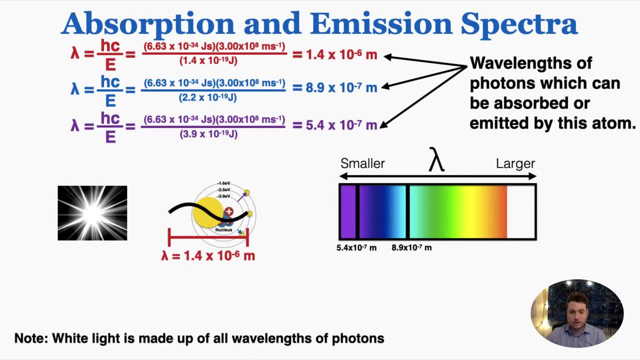 the black line, because this wavelength of 1.4 times 10 to the negative sixth meters would also be absorbed by the atom. Finally, photons of very long wavelength would pass through and complete the chart. So we call this an absorption spectrum. An absorption spectrum shows the spectrum of 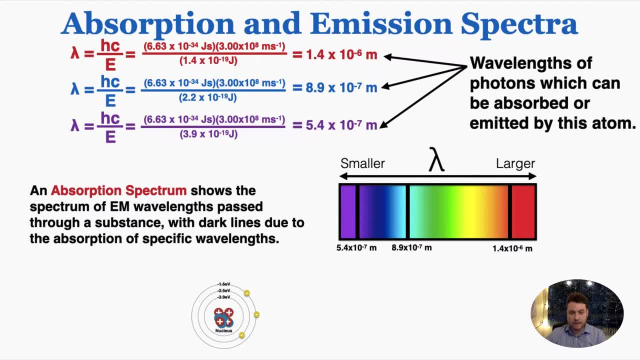 electromagnetic wavelengths pass through a substance, a collection of atoms with dark lines due to the absorption of specific wavelengths. So if I had a large amount of atoms of the substance and I passed electromagnetic waves of every possible wavelength through the substance and measured which wavelengths came out the other side, 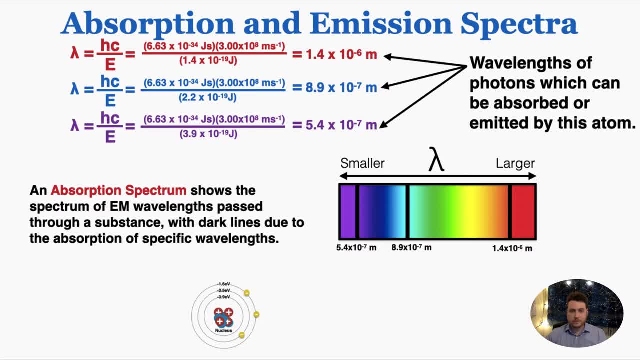 almost all wavelengths would make it through the substance, but there would be a few very specific wavelengths that would not make it through. that would cause black lines to appear on my diagram. I would call this diagram an absorption spectrum for this specific atom. We can now imagine that we have atoms of the same element. 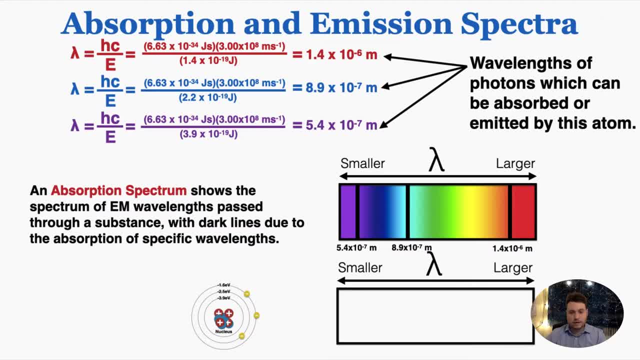 and this time we can place them in total darkness and see if we can measure any of the photons being emitted by the element. So I know that if electrons in this element were to lose energy, they could emit a photon of 5.4 times 10 to the negative 7th meters. 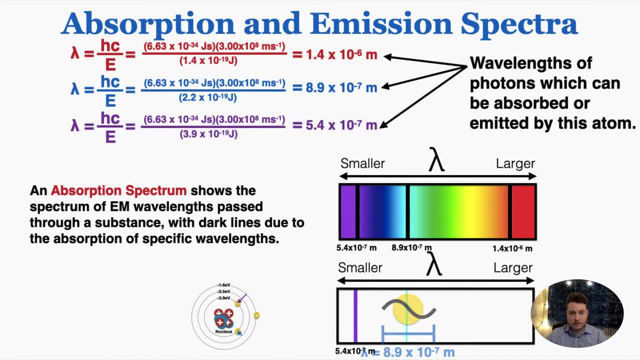 and a photon of 8.9 times 10 to the negative 7th meters and a photon of 1.4 times 10 to the negative 6th meters. So those would be the three places on my chart where I would detect photons. 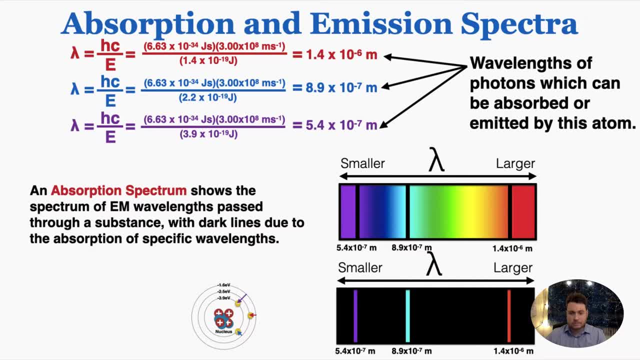 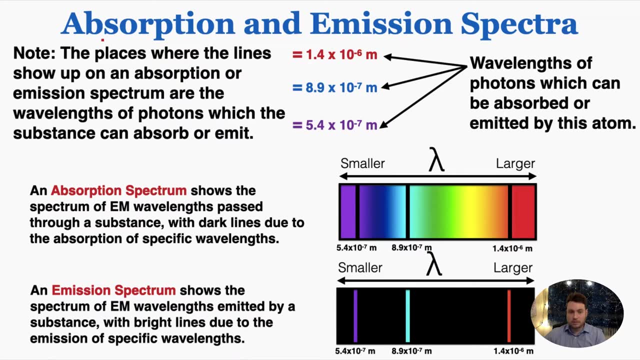 Everything else would be black. There wouldn't be any other EM waves hitting this chart. So we would call this an emission spectrum, because this shows the spectrum of electromagnetic wavelengths emitted by a substance with bright lights. You can see that the places where the lines show up on an absorption or an emission spectrum. 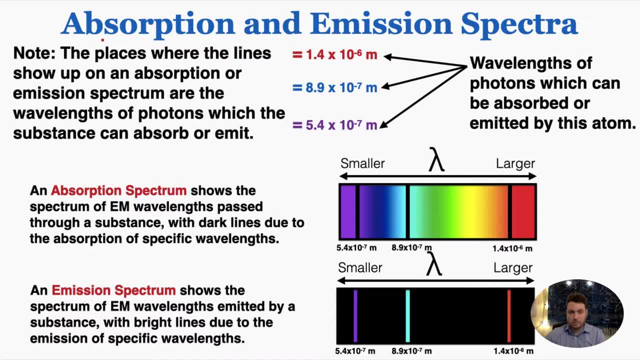 are the wavelengths of photons which the substance can absorb or emit. In the last lecture we learned how to find the energy frequency and wavelength of any photon that an atom can absorb or emit, And here you can see that these spectra diagrams show us those wavelengths that the atom can absorb or emit. 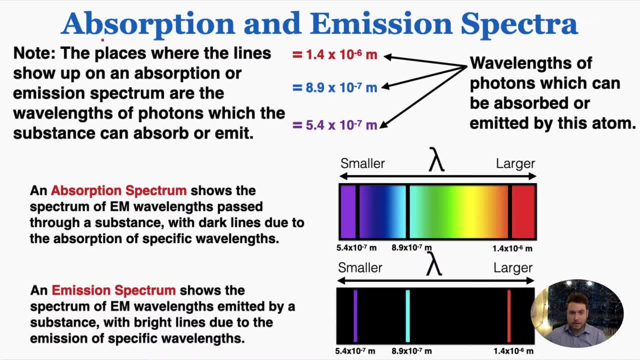 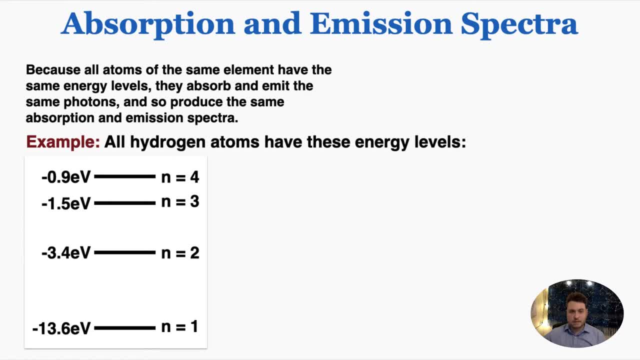 physically showing up on a chart we can make of all possible electromagnetic waves passing through or emitted from the substance, Because all atoms of the same element are emitting and all atoms of the same element have the same energy levels. they absorb and emit the same photons. 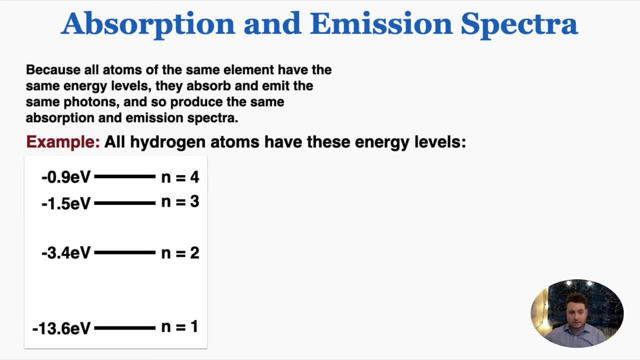 and so they produce the same absorption and emission spectra. So, as an example, all hydrogen atoms have these energy levels that I've listed here. I can run through and find all the possible energies of the photons that could be absorbed or emitted by a hydrogen atom. 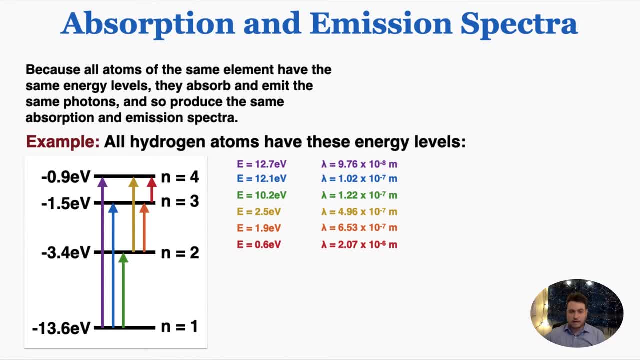 And I'll use the equation to find the wavelength. This is what I get when I do that. So if I fill in an absorption or emission spectrum using these wavelengths, it's going to look something like this: This is not drawn exactly to scale. 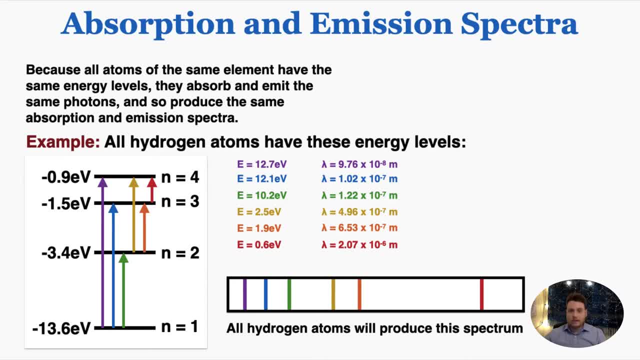 But because all hydrogen atoms have the exact same energy levels, they all have the same possible energy changes, which means they all emit or absorb the exact same photons with the same energies and the same wavelengths. So every single time you make an absorption or emission spectrum of a hydrogen atom, 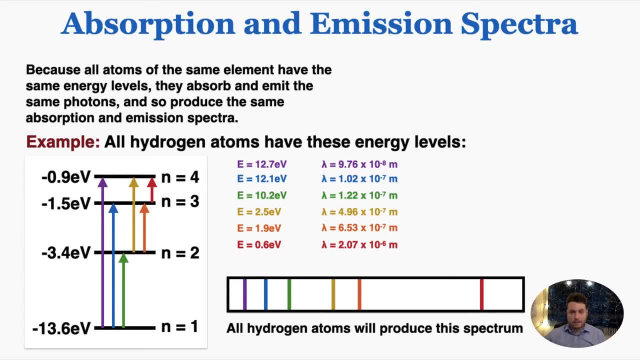 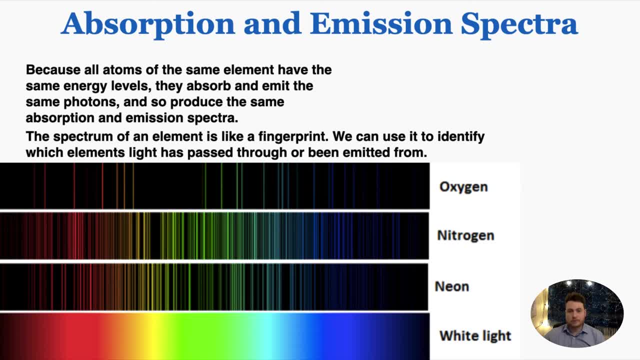 it's always going to look exactly the same, something like this, with the wavelengths in the exact same spots. The spectrum of an element is like a fingerprint that we can use to identify which elements light has passed through or been emitted from. As an example, these are the emission spectra of different common elements. 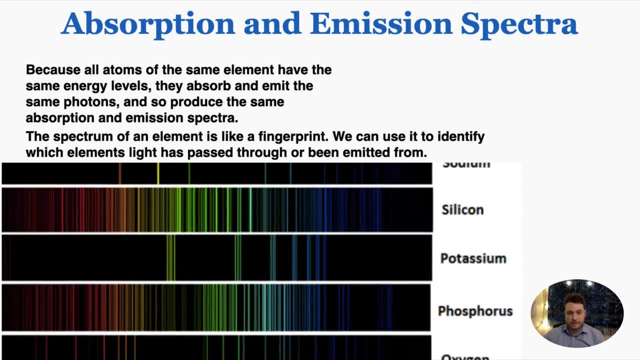 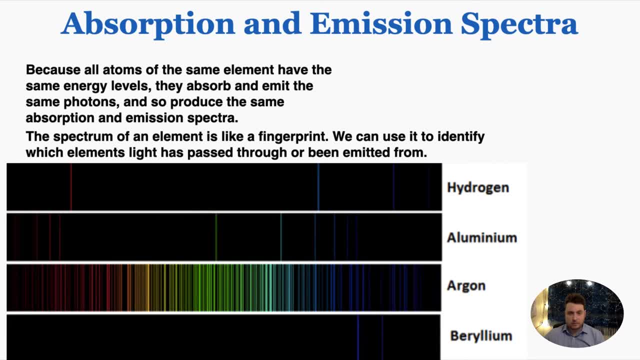 I'm just going to roll through and you can see how each one is kind of like a fingerprint for that element. We can always identify which element we're seeing in an emission spectrum because we already know what that element's spectrum looks like. So if we're given an emission spectrum, 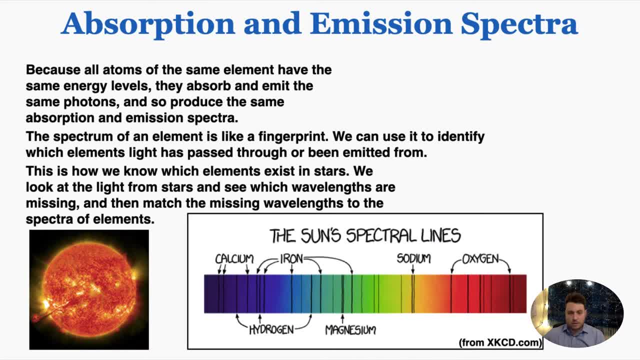 we can just match it up with the correct element. This is actually how we know which elements exist in stars. We look at the light from stars and see which wavelengths are missing, and then match the missing wavelengths to the spectra of elements. So this is how we know the chemical composition of the entire universe. 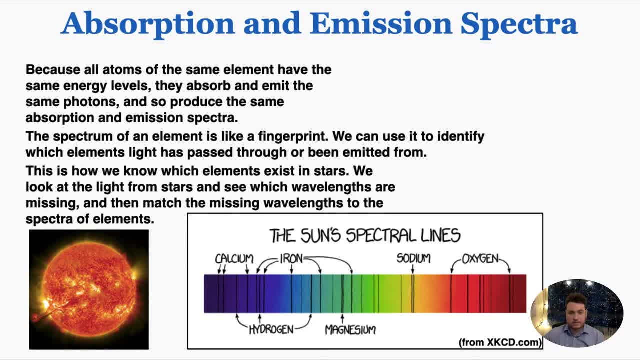 You can see in the picture that I've posted that this is the sun's absorption and you have all these different fingerprints of elements kind of superimposed on top of each other and we can just pick up the individual patterns and say, okay, this set of wavelengths is produced by hydrogen. 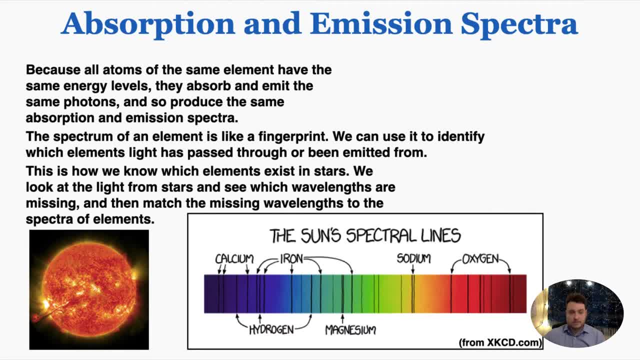 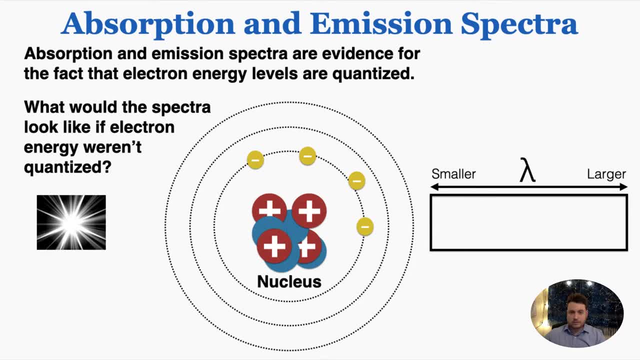 this is produced by iron, by calcium, by magnesium, etc. So this is how we know the exact chemical composition of the sun and all stars that exist in the universe. This next idea is really central to the topic. This gets asked about a lot on tests. 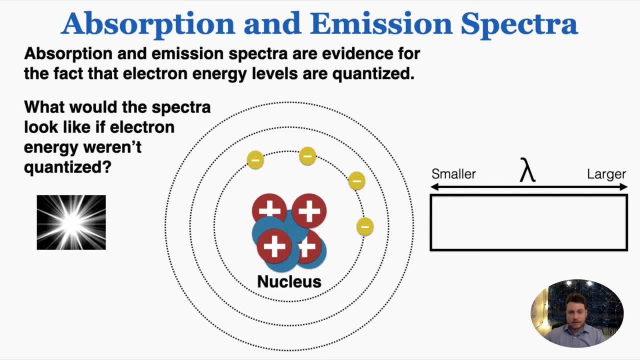 Absorption and emission spectra are evidence for the fact that electron energy levels are quantized. We can understand why by asking what the spectra would look like if electron energy were not quantized. This would mean that, instead of existing at very specific energy levels, 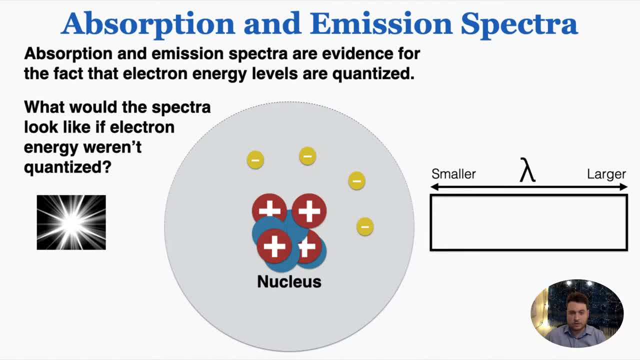 electrons could exist at any level of energy around the nucleus. It's difficult to say exactly what would happen here, because we would live in a very different universe if this were true, But one thing that would happen is because the electrons are able to exist at any energy level. they can now absorb any wavelength of photon. 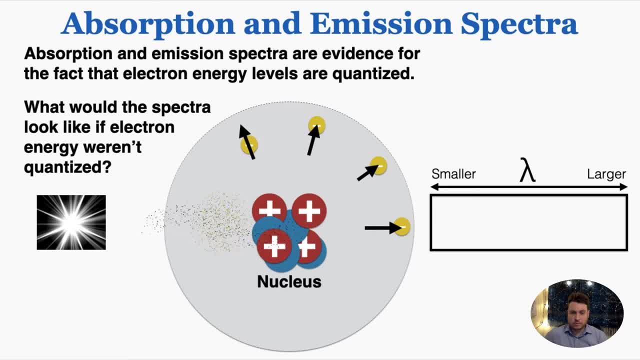 So any and all wavelengths could be absorbed by these electrons. So it could be that the spectra would just be black all the time. It could also be that maybe after reaching a certain limit of energy intake and maybe when all the electrons have escaped the nucleus. 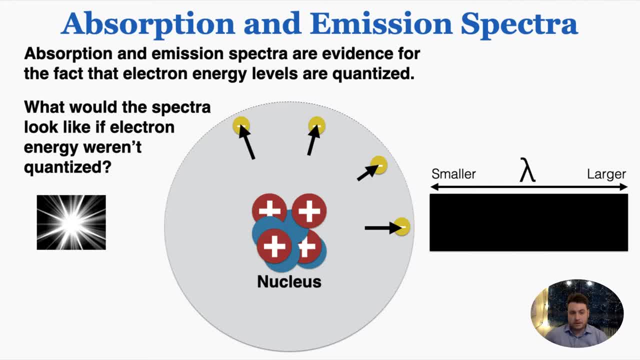 because they've gained so much energy. whatever photons just happen to randomly be left could pass through the nucleus and pop up as random lines on our chart. I would imagine that if the same thing happened again- because those wavelengths are random- this would result in different wavelength readings on the chart. 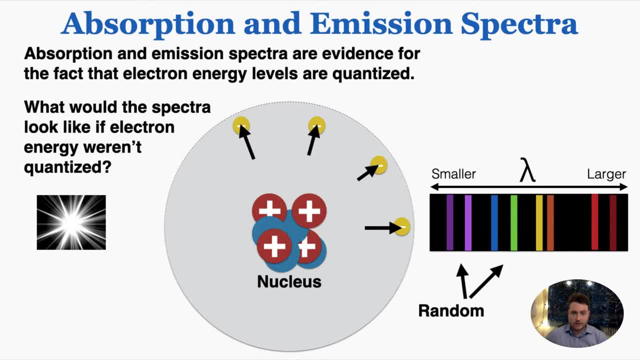 So instead of getting the same fingerprint every time for each element, we would get just random lines in random positions. This is probably not what would actually happen, and it's probably just a matter of time before a professional physicist hops into the comments and tells me that I am wrong. 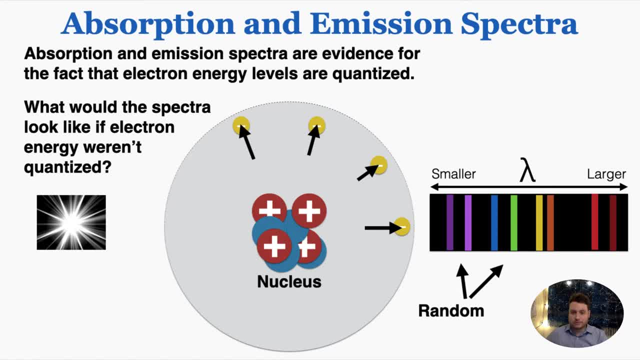 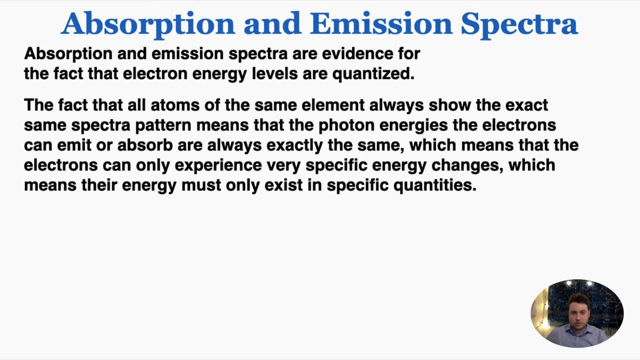 and something different would happen. But we don't live in that universe, so that doesn't really matter so much. What does matter is that the one thing that would not happen if energy levels weren't quantized is the exact same absorption and emission lines showing up for every single atom of the same element. 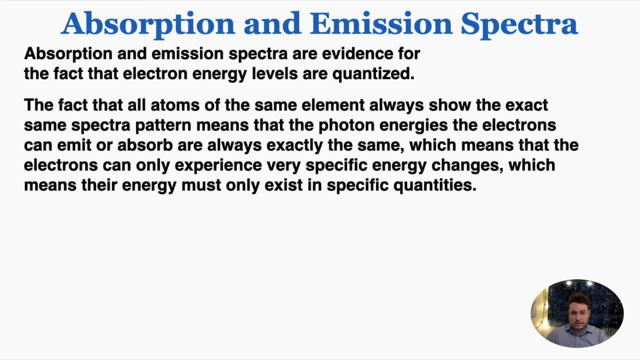 The fact that all atoms of the same element always show the exact same spectra pattern means that the photon energies the electrons can emit or absorb are always exactly the same, Because if it's always the same wavelength that's absorbed, it's always the same photon energy that's absorbed. 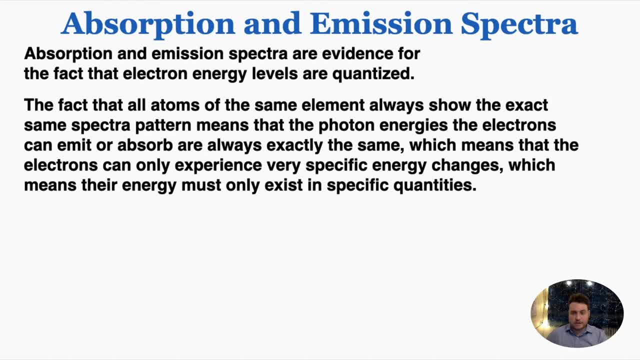 And this means that the electrons can only experience very specific energy changes, which means their energy must only exist in specific quantities and cannot exist between those quantities. So again, if we have the same spectra for all atoms of the same element, that implies that the same wavelengths of photons 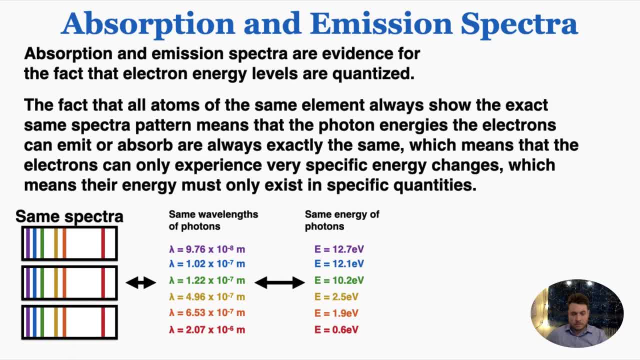 are absorbed by every single atom of the same element, which means the same energy of photons is absorbed, which means the electrons in each atom of the same element can only change energy by the same specific amounts, which means that the electron energy is quantized. 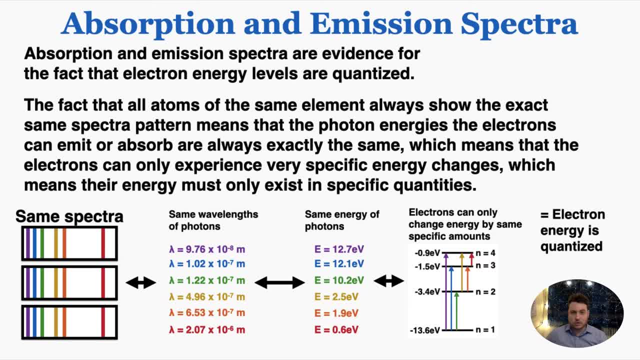 It can only exist in these very specific amounts and cannot exist between them. If it could exist between them, then we would get additional wavelengths that were absorbed or emitted, And that's not what we see in the real world. We always see the exact same spectra patterns. 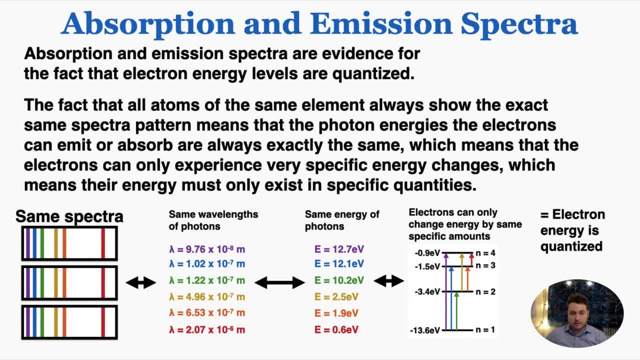 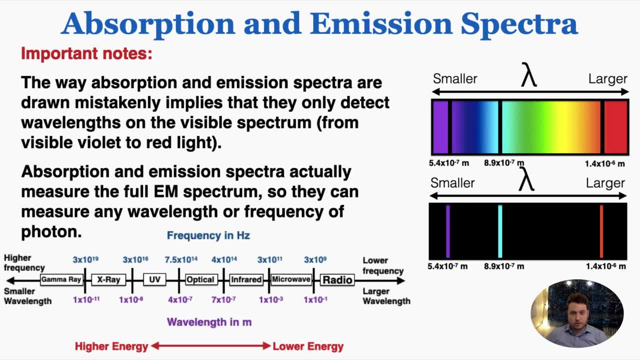 for all atoms of the same element. So this is how we know that electron energy is quantized. So absorption and emission spectra are evidence that electron energy is quantized. Just a few important notes to finish up the lecture. The way absorption and emission spectra are drawn. 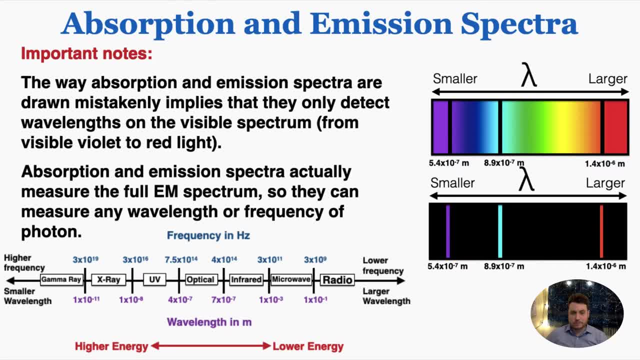 mistakenly implies that they only detect wavelengths on the visible spectrum, from visible violet to red light. They're very often drawn as rainbows, like what I've drawn here, Which implies that they only deal with visible light, but absorption and emission spectra actually measure. 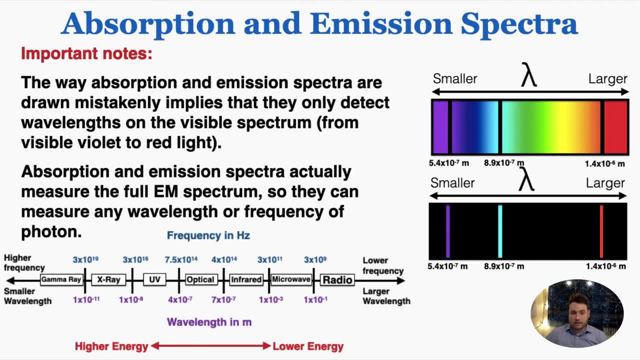 the full electromagnetic spectrum so they can measure any wavelength or frequency of photon. And remember visible optical light is only one very small part of the much larger electromagnetic spectrum, Because all photons with the same wavelength also have the same frequency. we can also draw absorption and emission spectra. 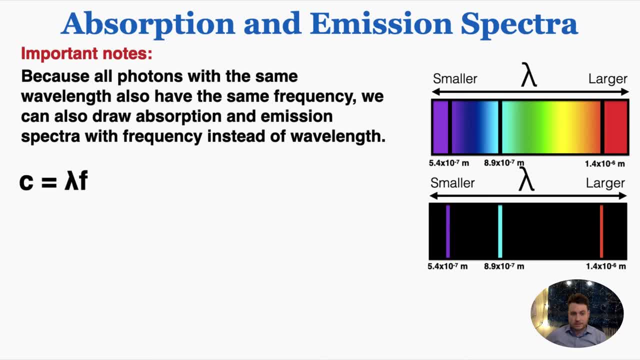 with frequency instead of wavelength. So because the speed of light is equal to wavelength times frequency, I can use this equation to solve for the frequency, along with the fact that this is the speed of light. So if I wanted to convert this into a frequency diagram, 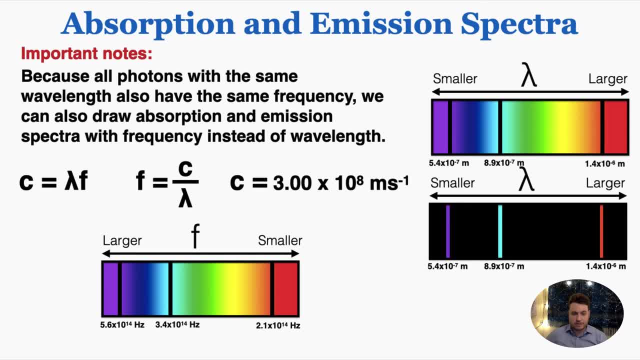 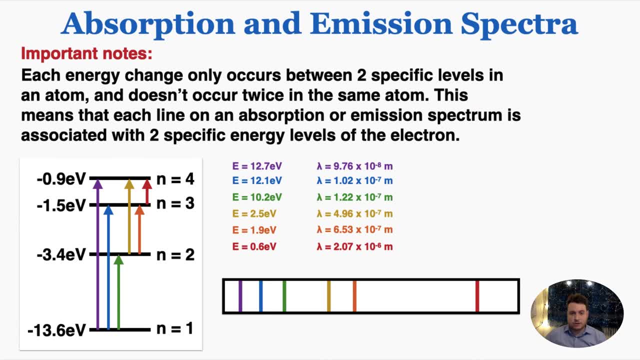 this is what it would look like. I just replaced all the wavelengths with frequencies instead, So we're also totally allowed to draw spectra with frequency instead of wavelength. This final note is hyper-specific, but each energy change only occurs between two specific levels in an atom. 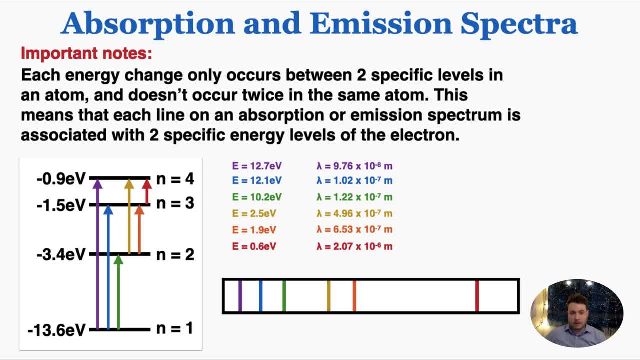 and doesn't occur twice in the same atom. This means that each line on an absorption or emission spectrum is associated with two specific energy levels of the electron, and only those two. So, as an example, these are six of the energy changes for hydrogen.